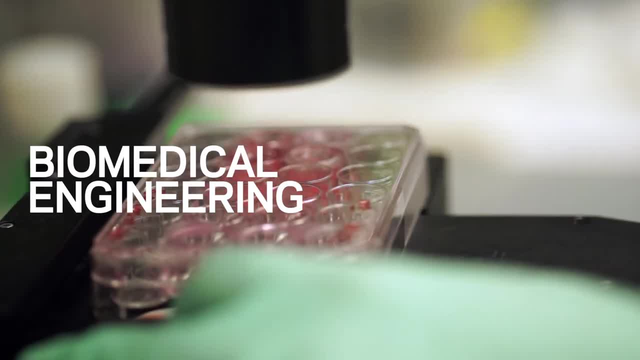 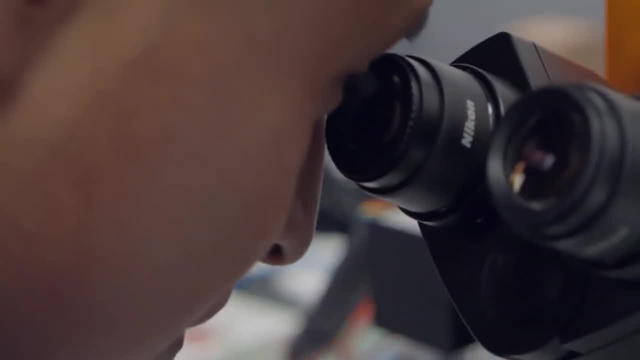 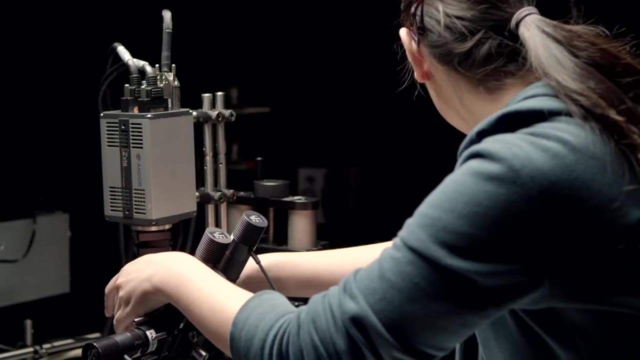 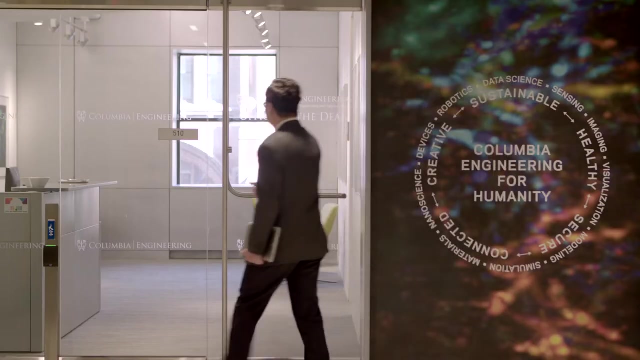 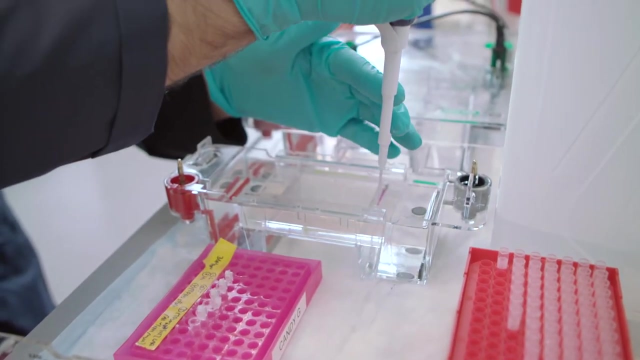 Biomedical engineering at Columbia University is highly interdisciplinary and encompasses research expertise across the whole university. Our department also emphasizes solving real life, complex biological and medical problems. In other words, engineering for healthy humanity. A biomedical engineer typically has a plethora of skills that span life sciences and biology. 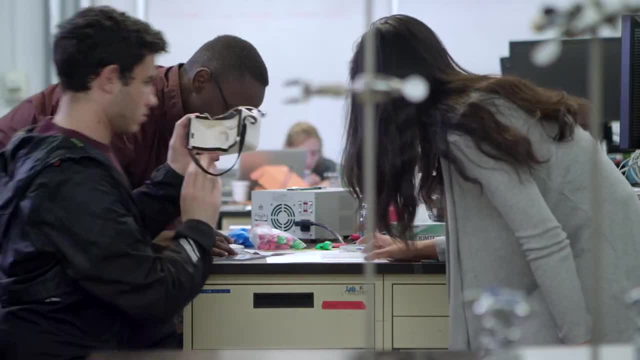 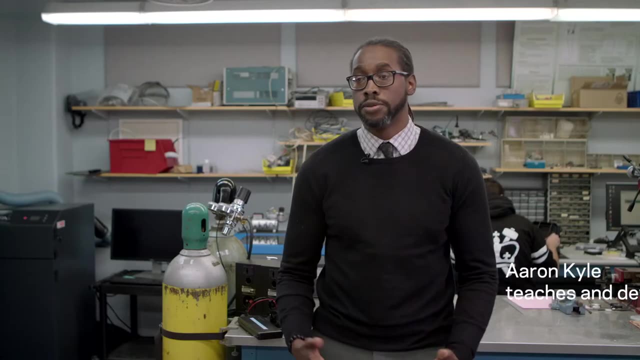 traditional engineering. Our people have to have an appreciation for socio-economical concerns, especially, say, our teams that are working in low resource settings. But all of our groups have to be cognizant of the entrepreneurial aspects. So a BME is a hybrid. 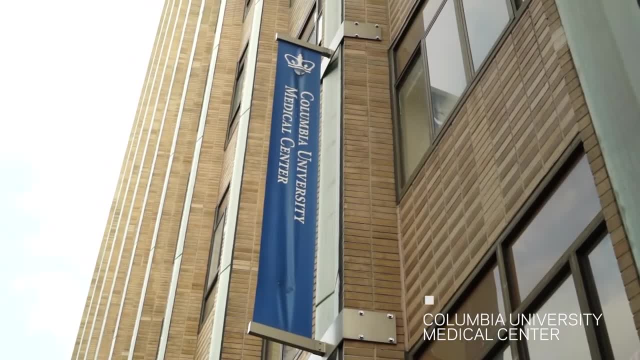 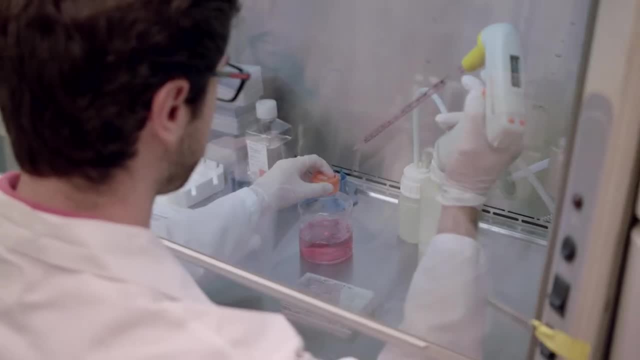 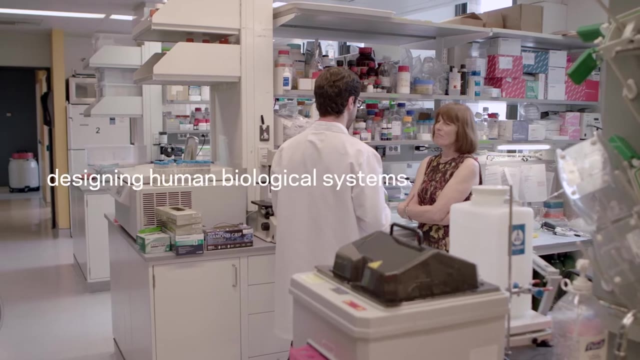 engineer. Columbia University is fortunate to have a top medical school, So it's an incredibly rich and diverse opportunity to cross-pollinate engineering principles with the needs of medicine. We're in a lab for stem cells and tissue engineering. We are now capable to repair organs and parts. 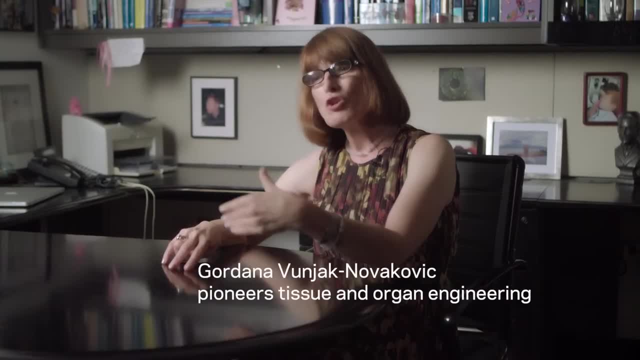 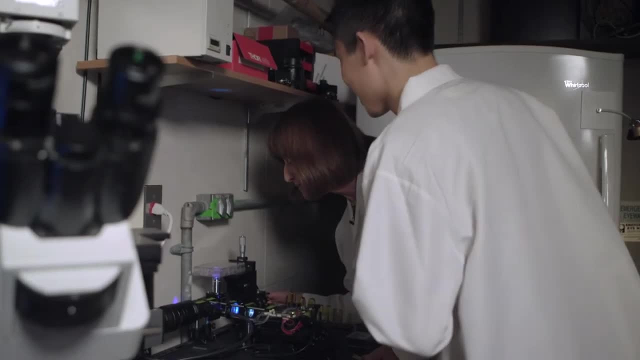 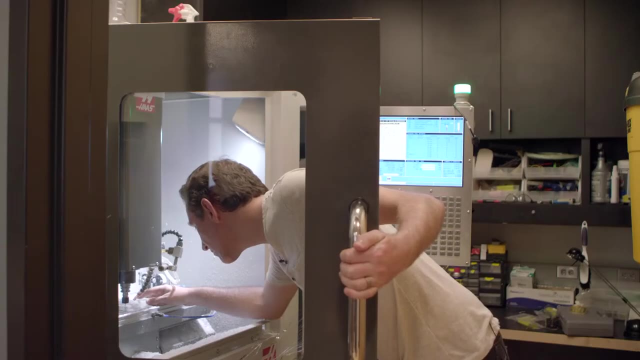 of the human body. We are becoming much more sophisticated now with our designs of the biological systems, So you can make a whole set of very small size organs and tissues from an individual on a chip And you can do testing in a patient-specific way. So 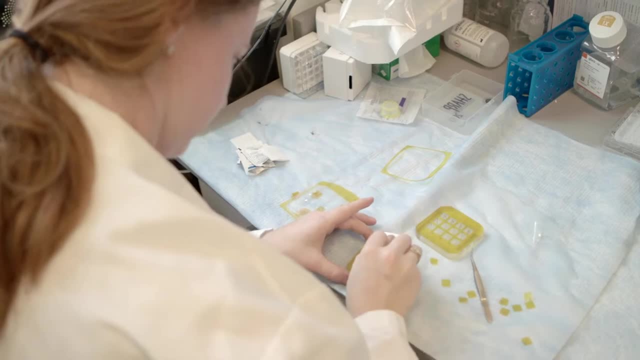 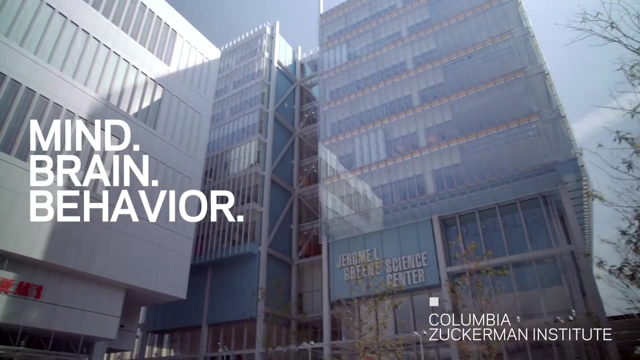 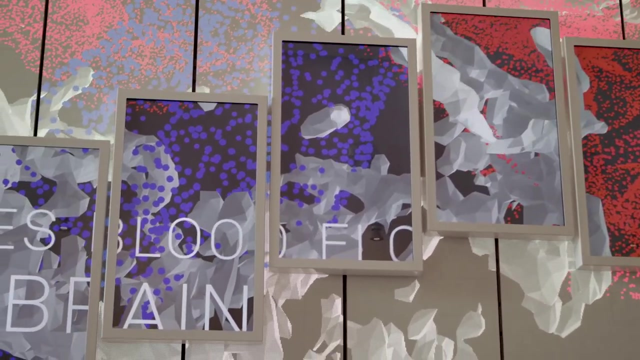 when we talk today about precision medicine, this is one of the most effective directions in which this area is going. I'm part of the Zuckerman Institute at Columbia. It's the Mind-Brain-Behavior Institute, and we're really trying to understand the brain from every possible angle. In my lab we develop 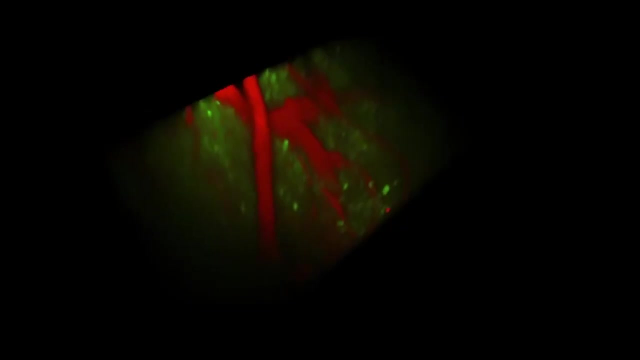 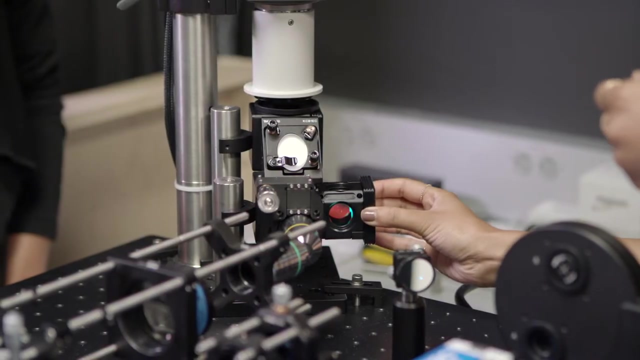 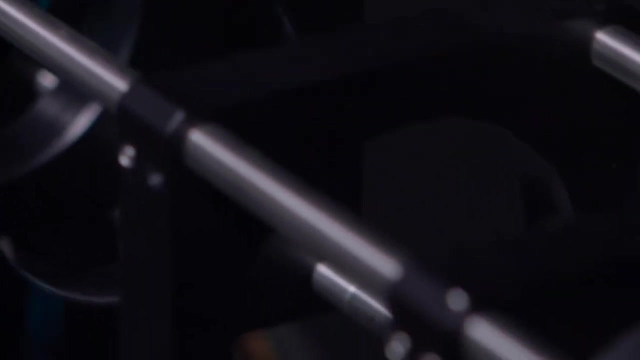 new microscopes and new ways to image the brain. Imaging, in particular biomedical imaging, really spans a huge range of disciplines And, quite uniquely I think, we extend our techniques quite often into studies of disease. So we're studying stroke, We're studying brain development, We're studying Alzheimer's.